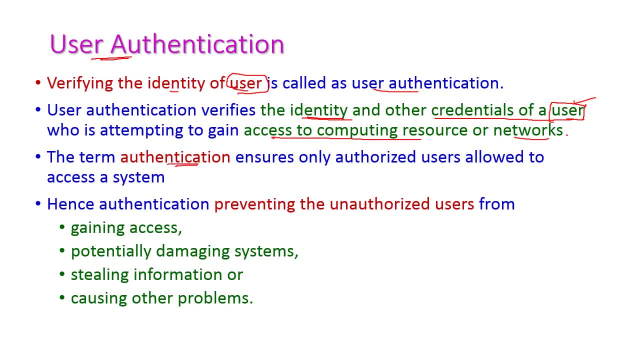 Okay, For that we can use this authentication Here, the authentication preventing the unauthorized users from gaining access to computer resources or preventing the potentially damaging the system, or preventing the stealing information or causing other problems, Because if we allow the unauthorized users to access our systems, we can face so many problems. 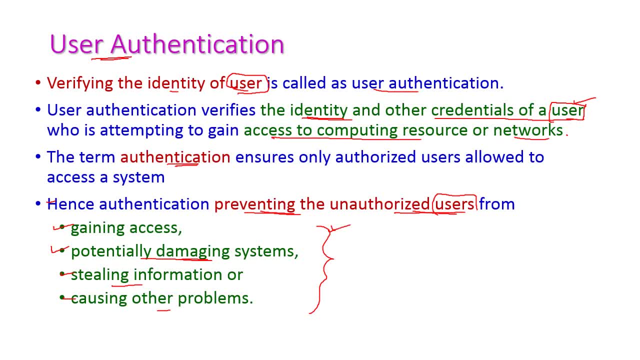 Okay, To overcome all those things, we have to authorize a particular person. Only those authorized person are allowed to access our system. For this we have to verify whether the person is authorized or not. Okay, For that we have to use this term: authentication, That is, user authentication. 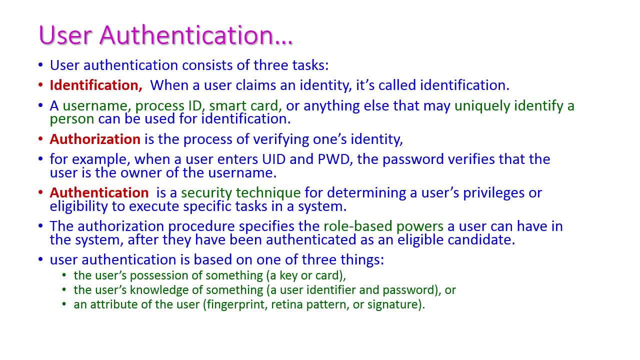 User authentication consists of three tasks. First one is identification, authorization and authentication. Let us see what is identification. Identification means when a user claims an identity is called as identification. The identity may be a username, a process ID, a smart card or any other thing which may be uniquely given to all the user, All the user- And these items can be used for the identification of user Right. And second one is authorization. Authorization means 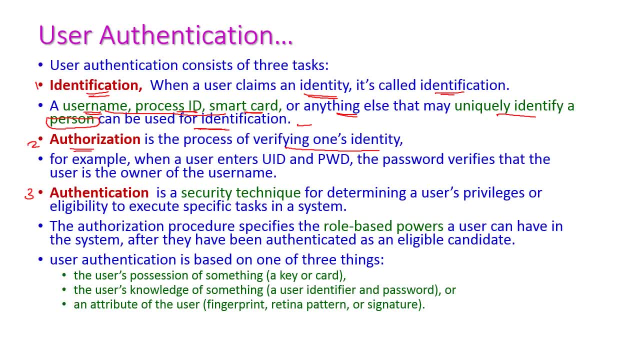 It is the process of verifying one's identity. Okay, Verifying the user identity is called as authorization. For example, when a user enters his own user ID and password, then the authorization will verify the password that the user enter: is the owner of the username or not? Okay, So verifying the user is called as authorization. 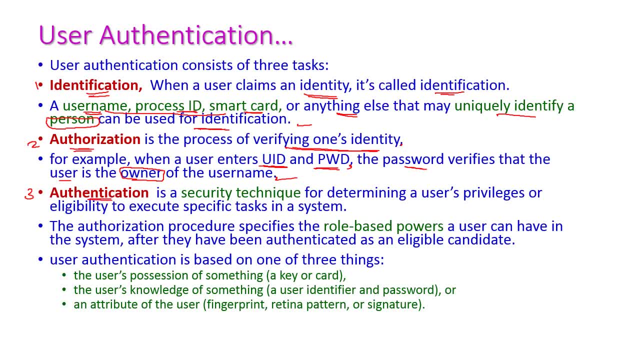 And second one is authentication. Sorry, The third one is authentication Here the security technique for determining the user's privilege or eligibility to execute specific task in the system. Okay, So this is called as authentication. That means the user, the particular user, is accessing the allocated resources, or not? Okay, That is called as authentication. That is authentication. 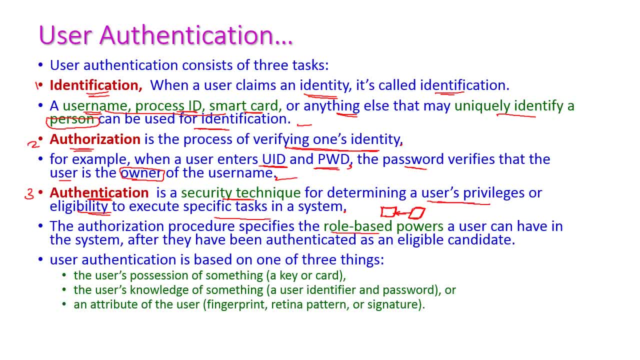 The authorization procedure specifies the role based powers a user can have in the system. Okay, What type of role the user is going to play in the system? Okay, After they have been authenticated on eligible candidate: Okay, Suppose if the person is allowed to take printer, that is, take printout on a printer, but the person is also trying to access the scanner. 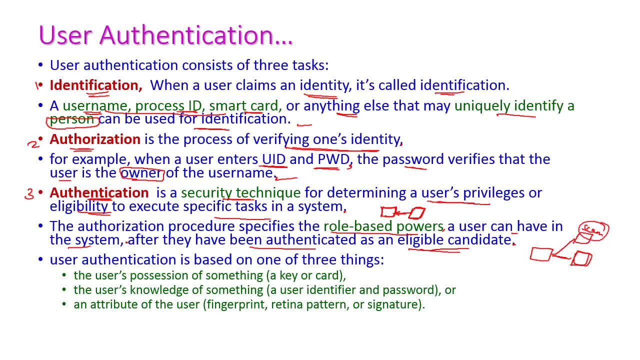 Then this is the unauthorized access Right. So the authentication will verify whether the person is accessing only the printer or not. Okay, So this is called as authentication. The user authentication is based on one of the three things. What are the three things? First one is the user's possessions of something. That is what the user is having the identity. 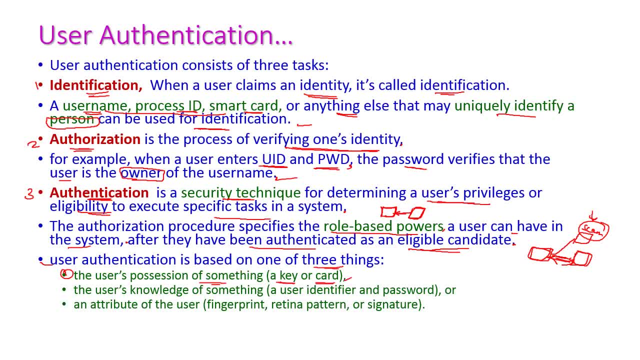 Okay, So the user has a key or ID card or whatever it may be The object used for identification. And second one, the user's knowledge of something. That means the user identifier, that is, user ID and password. Okay, User ID and password, that belongs to user's knowledge. And the third one is an attribute of the user. Attribute of the user means biometric authentication. 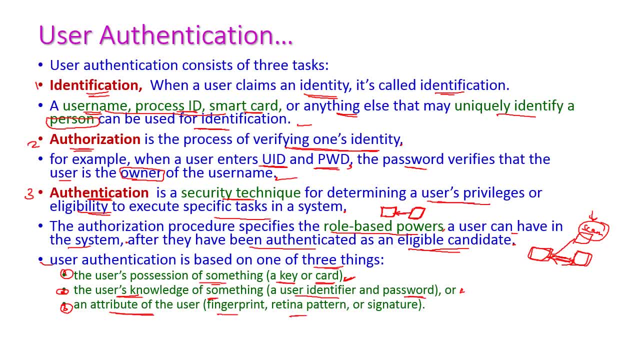 Okay, Fingerprint retina, that is I retina retina printer and the signature. everything will be come under the attribute of user. okay, that is the user's object, user's knowledge, that is, user id and password, and third, one is user's attribute. by using these three, the authentication will verify the user is authorized user or not. 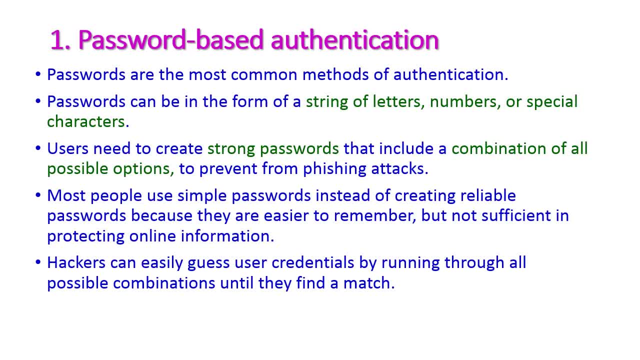 password based authentication. passwords are most common methods of authentication. that is all. the users are allowed to create their own password and, based on the password, the authentication will verify whether the given user ID and password are belongs to the authorized user or not. okay, and the passwords can be in the form of string of characters, numbers and special. 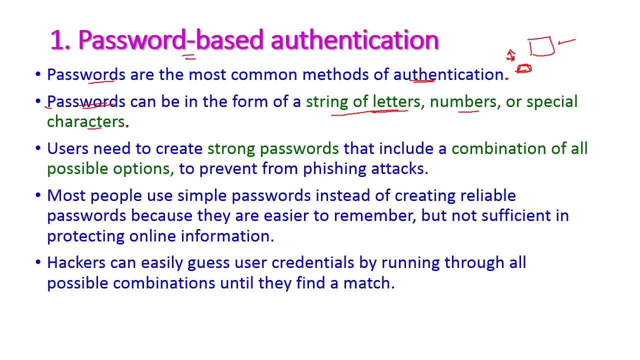 characters: okay, and the strong password means the combination of letters, numbers and special characters: okay, all the users are asked to create only the strong password. then only the information, that is, the sensitive informations, will be prevented from the attackers. they can try the phishing attack- okay. phishing attacks means the hacker will try all the possible combinations of password until they. 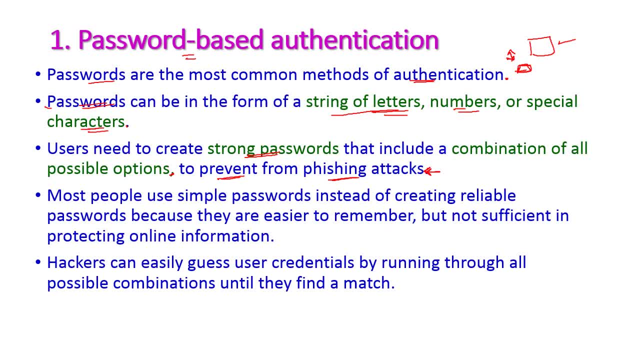 find the password. okay, and then they can try the phishing attack. okay, and then they can try the phishing attack. okay, and then they can try the phishing attack. okay, and then they can try the correct password. but most of the people use only the very simple password instead of creating a. 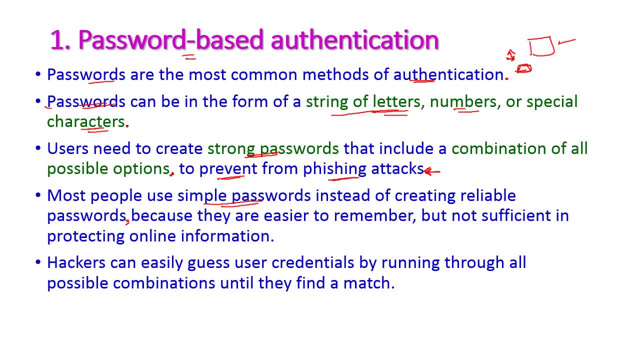 reliable password, because the simple passwords are easy to remember. but this is not sufficient in protecting online information. those information may be very sensitive, and here hackers can easily guess the user's credentials by running all possible combinations of password until they find a match. So users have to create the strong password. Multi-factor authentication, which is: 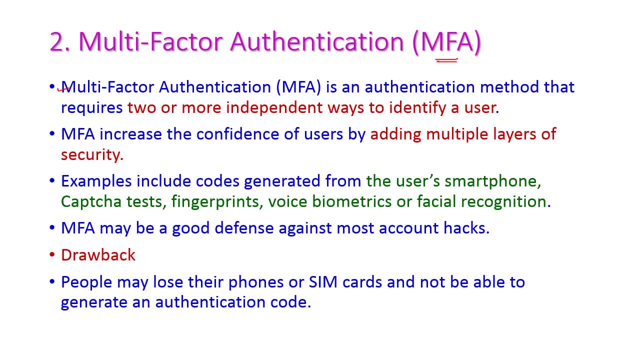 otherwise called as MFPA, and it is another important authentication method which requires two or more independent ways to identify a particular user. That is, apart from user ID and password, the user have to enter another identification for verifying the user. Hence the MFPA increase the confidence of user by adding multiple layers of security. 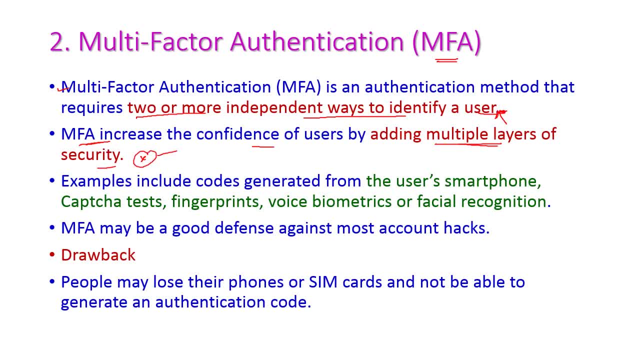 By adding multiple layers of security. What is the other layers, apart from user ID and password? The code generated from user's smartphone CAPTCHA test fingerprint, voice, biometric or facial recognition. Okay, So hence the MFPA, that is, multi-factor authentication, is very good method, which will 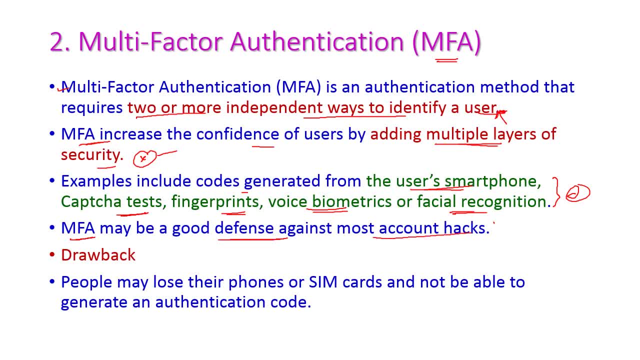 defense against most account hack. Hacking the account is somewhat difficult in this MFPA And this is also having some drawback, that is, people may lose their phone or SIM cards, hence they cannot be generated the authentication code. This is the drawback of 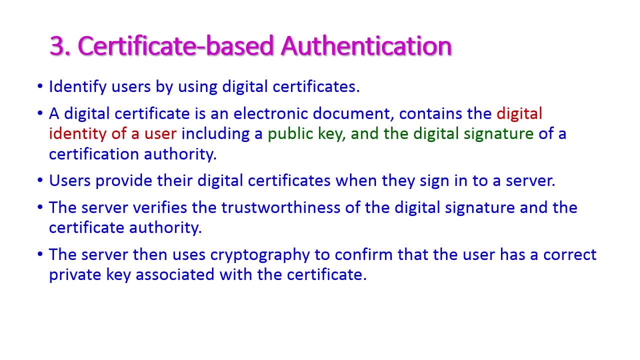 M, F? a. that is multi-factor authentication. The next one is certificate based authentication, which is used to identify the user by using digital certificates. Okay, Everyone user have to produce the digital certificate for entering into the system, right? This digital certificate is an. 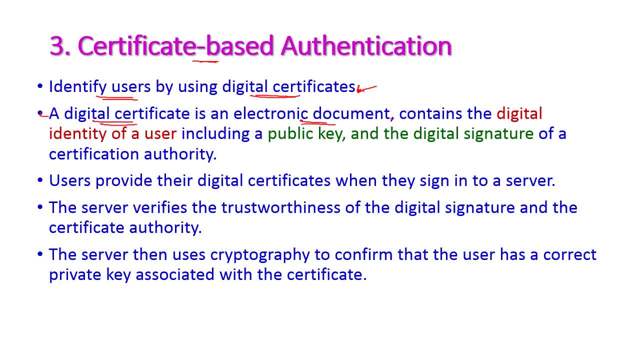 electronic document Doctrine for Makeанд b. The digital identity of the user. okay, since this identity contains the public key and digital signature of certificate authority, Here the certificate authority who will provide the public key and private key for the users? that is, unique private key for all the users. 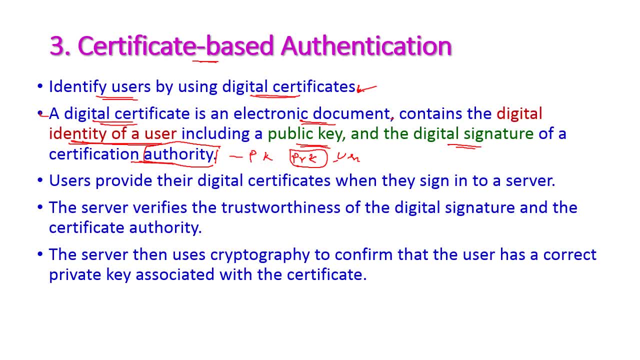 A common public key and unique private key for all the users And in the digital certificate it is having the public key as well as the digital signature of certificate authority right. The user have to provide their digital certificate whenever they sign into the server. 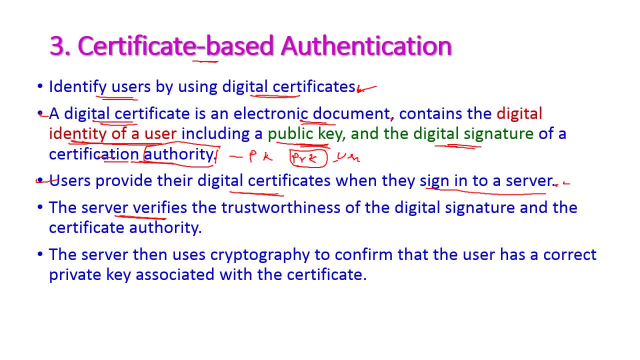 Okay, now the server verifies the trustworthiness of the digital signature, because the digital signature contains the public key and the digital signature of certificate authority, isn't it? So the server will get Verify those two things and it will conclude that, whether the user is authorized user or not, okay, 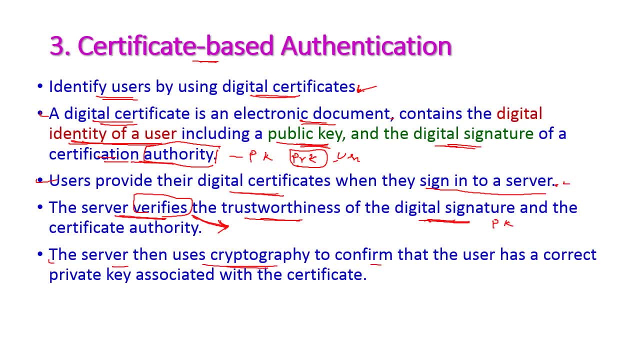 The server then use cryptography to confirm that the user has a correct private key associated with the certificate or not. okay, So for all the user, they are having their own private key. The private key is provided by the certificate authority only. okay. 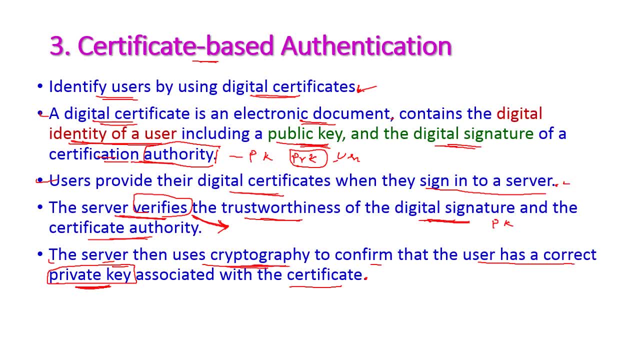 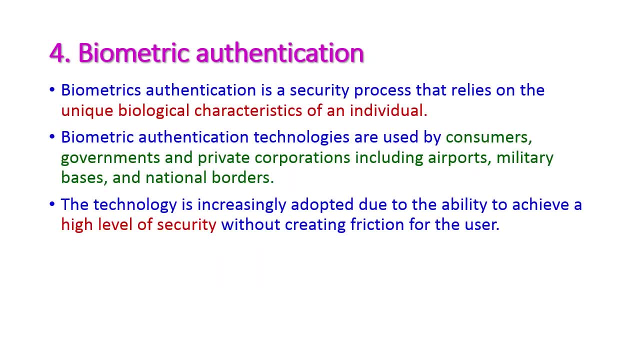 So the server Use cryptography to confirm that the user has correct private key associated with this certificate. Biometric authentication: This is a security process that relies on unique biological characteristics of an individual. This is important. okay, Every person is having its own unique biological characteristics. 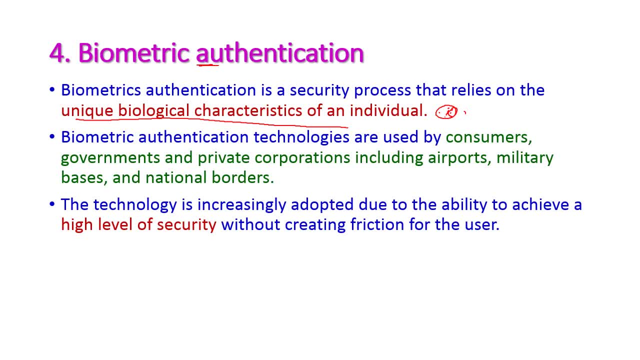 For example, the fingerprint and the iris pattern, etc. So based on those biological characteristics, the particular user is being identified. okay, So this biometric authentication technologies are used by consumers, governments, private corporations, which includes airport, military and national borders. 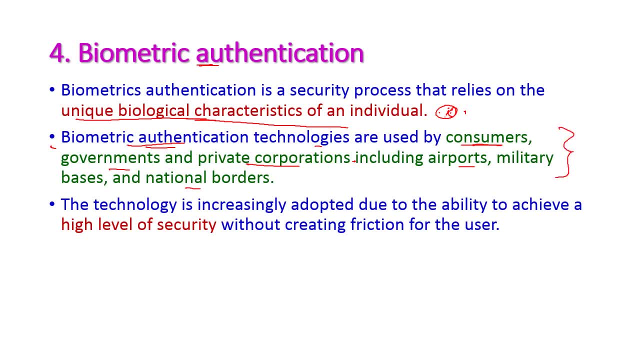 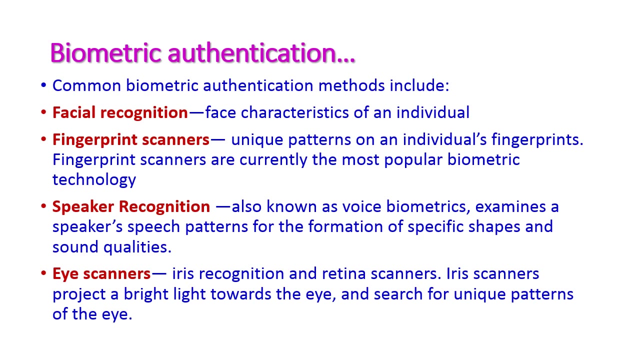 Nowadays, almost everybody are using this biometric authentication. okay, because this will provide a high level security without affecting the user. okay, Because only the particular user has is having its own biological identity. The common biometric authentication methods includes the facial recognition, fingerprint scanner, speaker recognition and the eye scanners. 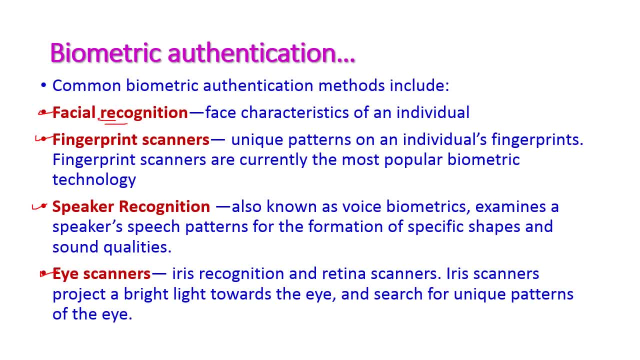 The first one is facial recognition, that is, the face characteristics of an individual. So each and every individual are having their own biometric facial characteristics And based on that we can identify the particular user, okay. And second one is fingerprint scanner. 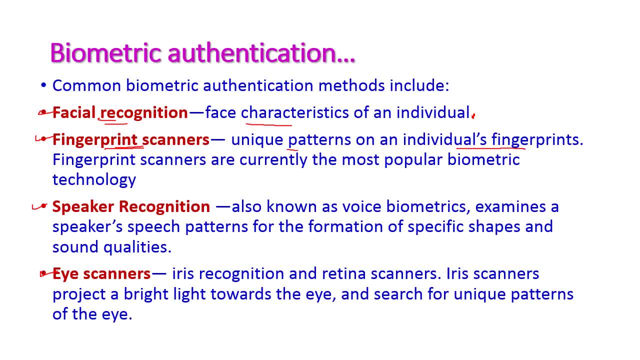 And this is the unique pattern of individual's fingerprint, correct? Nowadays the fingerprint scanners are very popular. And the next one is speaker recognition, which is known as voice biometric. okay, So this authentication examines the speaker's speech pattern. 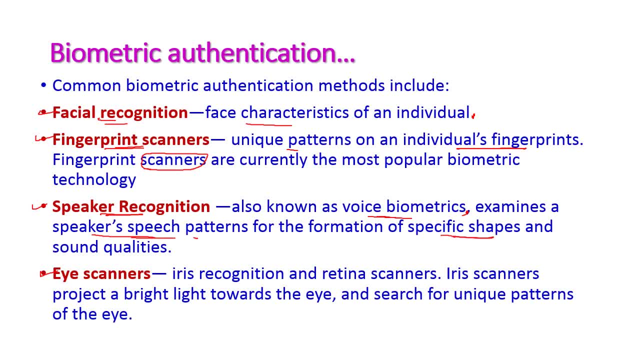 For the formation of Specific shape and sound qualities, how the particular user is going to speak. okay. And third- that is the last one- is scanners: eye scanner. Eye scanner is for iris recognition and retina scanner. Here a bright light will be projected on eye and search for unique pattern of a particular user's eye. okay, 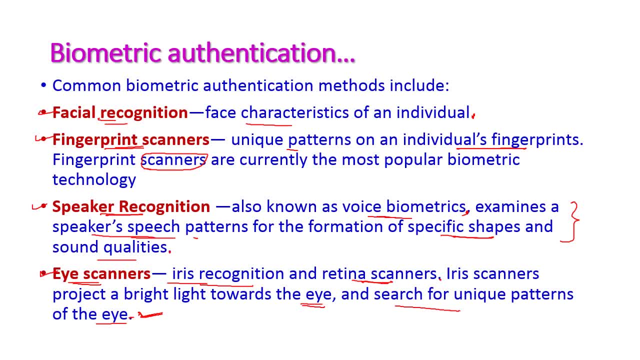 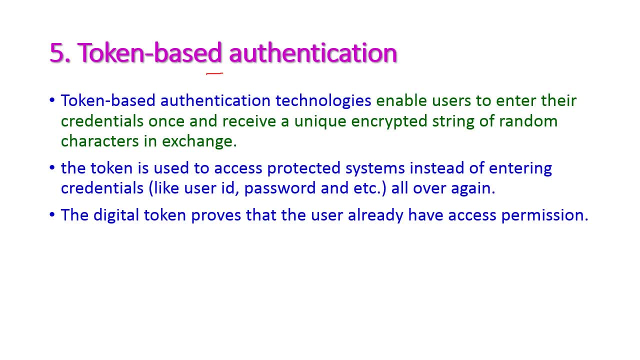 And based on that, this authentication method can Verify the particular user. The token-based authentication: This technology enables user to enter their credentials once and receive a unique encrypted string of the random characters in exchange. Okay, once they enter all those details, then immediately they will get an encrypted string. 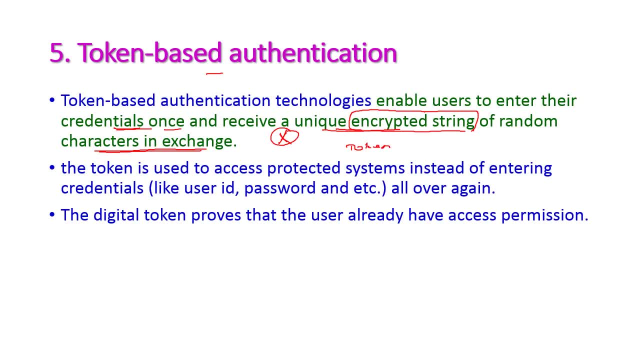 Then this is called as token. Okay, and this token is used to access the protocol. This is a protected system. instead of entering all the credentials- that is, user ID, password and other details- again and again- See once they have entered and the system will create an encrypted text and this is called as token. okay.